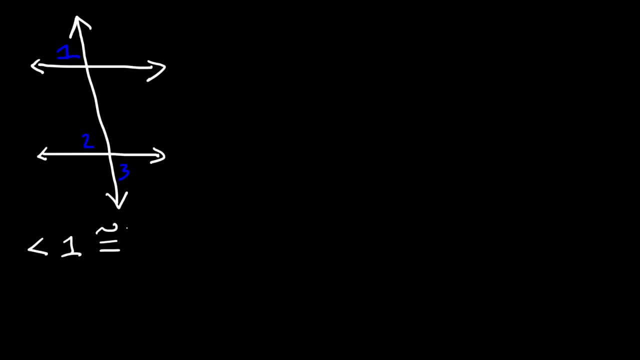 given that angle 1 is congruent to angle 2.. Our task is to prove that angle 1 is congruent to angle 3.. So how can we do it? Well, let's start with a two column proof. In the first column, we're going to write all of our statements, and in the second column, we're going to write: 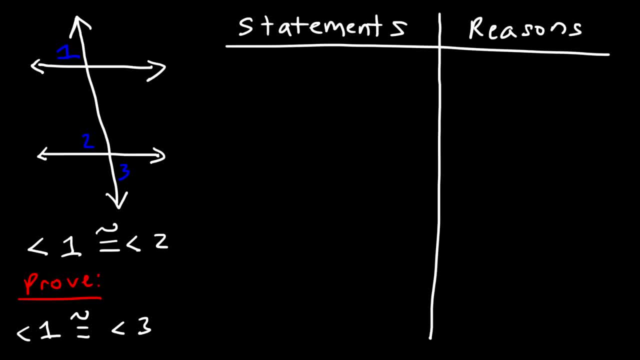 the reason. So the first thing you want to write is what you're given, That is, angle 1 is congruent to angle 2.. So that's statement 1.. Now what else can we say? Whenever you have two lines intersecting each other, they form vertical angles. So let's say, if this angle is 60,. 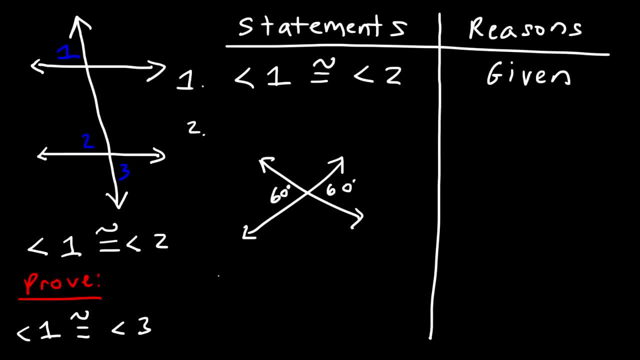 this angle is 60 as well. So notice that angles of angle 2 and 3 are vertical angles. We can say angle 2 is congruent to angle 3.. And the reason: Vertical angles are congruent. Now, if angle 1 is congruent to angle 2 and if angle 2 is congruent to angle 3, we can: 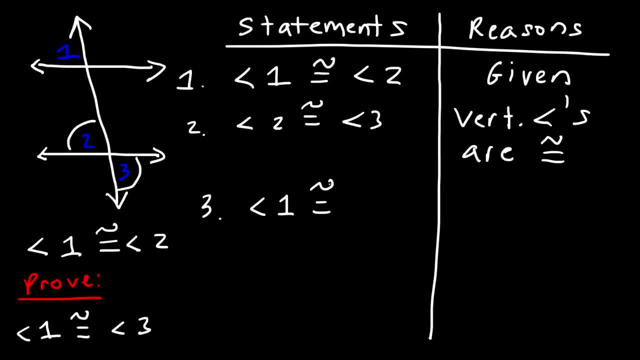 make the statement that one is congruent to angle three, and this is based on the transitive property. so another example of the transitive property is if angle a is congruent to angle B and if angle B is congruent to angle C, then we could say that angle a 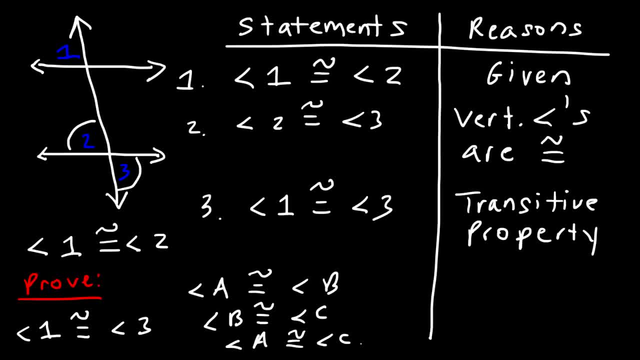 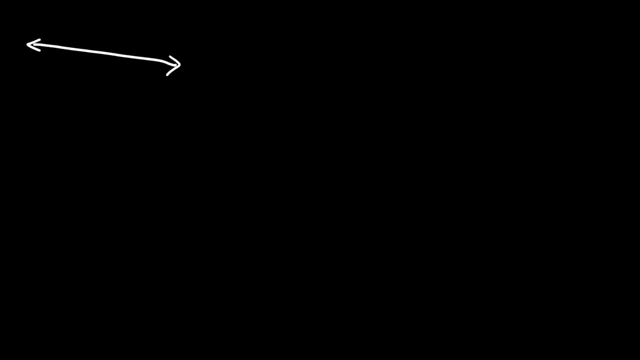 is congruent to angle C. so that's the basic idea of the transitive property, especially as it relates to angles. so that's it for this problem. now let's look at another example. so let's call this angle one, angle two, angle four and angle three. let's say that we're given that angle one is. 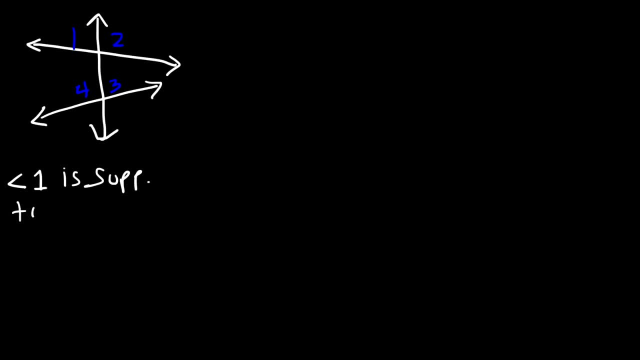 supplementary to angle two, and also angle three is supplementary to angle four, and also angle one is congruent to angle four. your task is to prove that angle two is congruent to angle three, so feel free to design a two-column proof that proves the statement. so if you want to pause the video- and now's the time to do it- 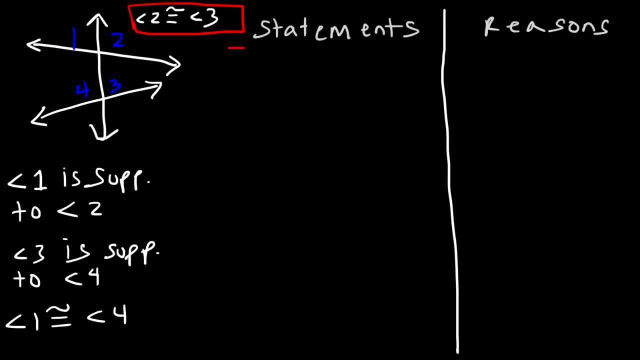 now the first thing we should do is write the statements that were given. number one: we're given that angle one is supplementary to angle two, so that's a given. number two were given that angle three is supplementary angle 4, so that's given as well. and also number 3: angle 1 is congruent to angle. 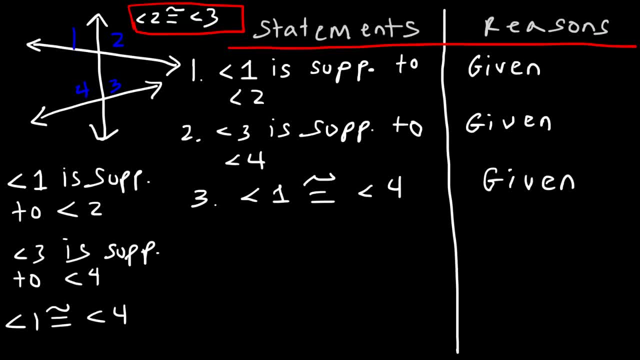 4. so that's given. so what can we do at this point? now let's use numbers. now we know that angle 1 and 4 congruent. so let's say, if angle 1 is 100 degrees, that means angle 4 is a hundred. now notice that one and two form a linear pair. 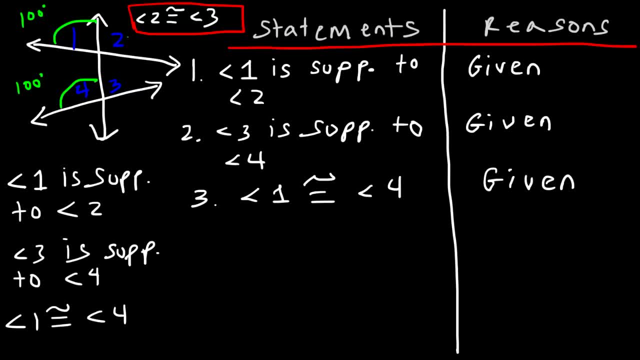 that means that the additive 180 they're supplementary. so if angle one is a hundred, angle two has to be 80, and if angle four is a hundred, and four and three form a linear pair, which means their supplementary angle three has to be 80 as well. so therefore we can make the statement that angle 2 is congruent. 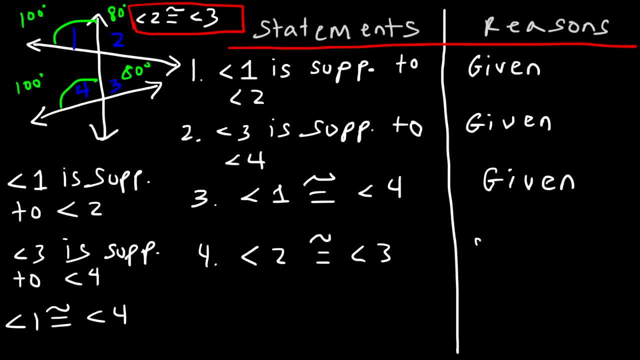 to angle 3, and the reason could be dicen from the reaction: if x sus STARdel imperial declines. Point c dr that supplements of congruent angles are congruent. Now let's see if we can make sense of that reason. So let's focus on a sentence. So what are the supplements? 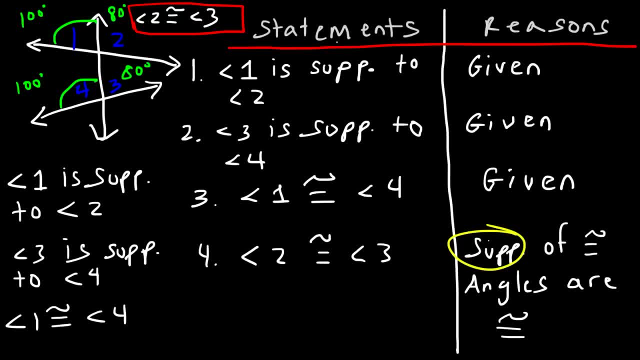 that are talked about in that sentence. The supplements are angle 2 and angle 3.. Angle 2 is supplementary to angle 1.. Angle 3 is supplementary to angle 4.. So the supplements, that is, angle 2 and 3 of congruent angles, the congruent angles. 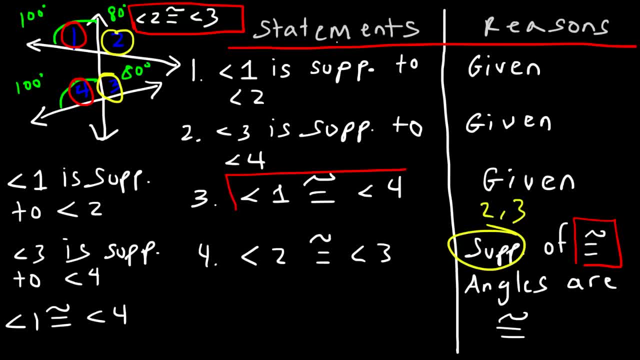 are 1 and 4, because in statement 3 we said 1 and 4 are congruent. So supplements 2 and 3 of congruent angles, which are 1 and 4, are congruent. So if 2: 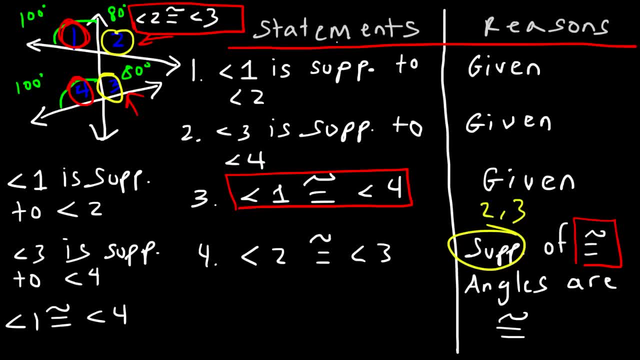 and 3 are supplements of these congruent angles, then two and three are congruent. That's what that sentence is saying. So hopefully that makes sense to you And that's how you can prove that angles two and three are congruent, because they're. 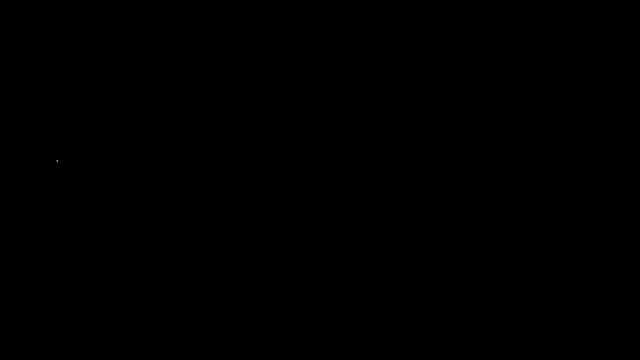 supplementary to congruent angles. Let's work on another problem. So this is going to be A, B, C and D. So this is going to be angle one, angle two, three and four. So, given that angle BAC is congruent, 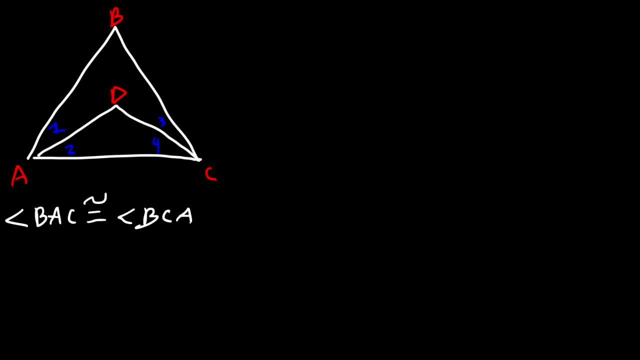 to angle BCA and that angle two is congruent to angle four. go ahead and prove that angle one is congruent to angle three. So you can try this out if you want. Let's start with a two column proof. So what's the first thing that we should write? 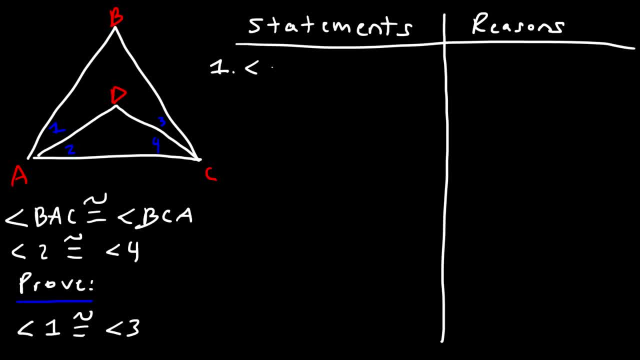 So we should always write what we're given, And that is, angle BAC is congruent to angle BCA, and that angle two is congruent to angle four. So that's given. Now what else do we know? The next thing that we need to do: 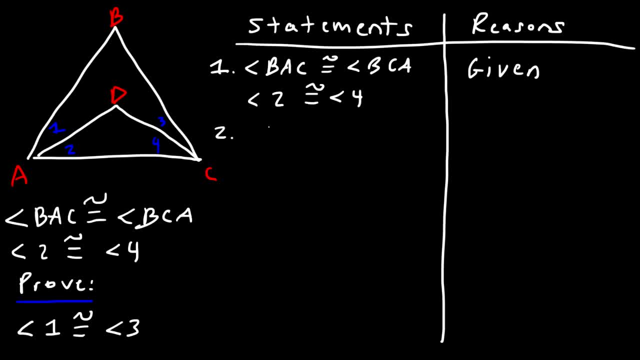 is make the statement that the measure of angle BAC is equal to the measure of angle BCA. We can say that the measure of angle two is equal to the measure of angle four, And the reason for this is the definition of congruent angles. 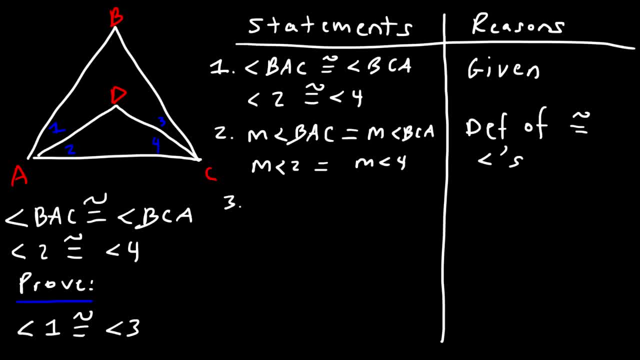 Now let's move on to step three. Notice that angle BAC is the sum of angles BAC and 2, and CCP is the sum of angles AAC and three. The BAC angle is congruent to Angles three and four, So we could say that: 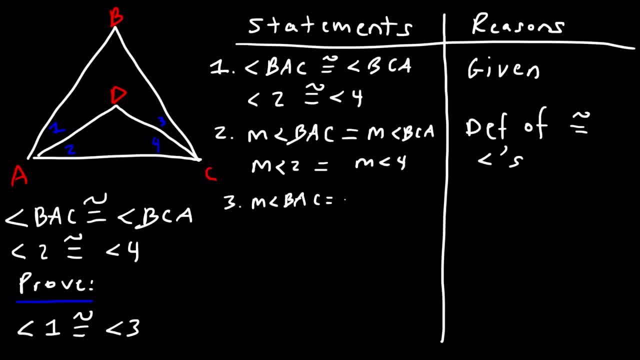 the measure of angle BAC is equal to the sum of the measures of angle one and angle two Of angles BAC and four. Let's dig this out a �P. We could also say that the measure of angle BCA is the sum of the measure of angle 3 plus. 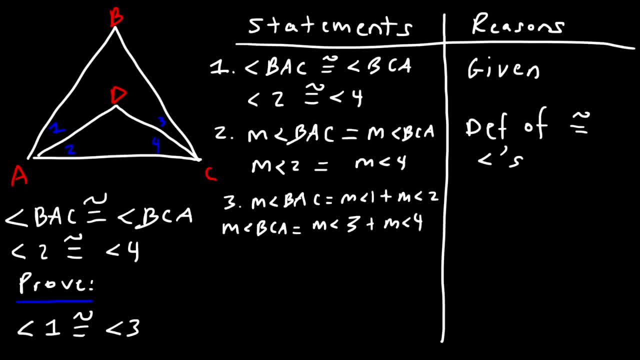 the measure of angle 4,, as we highlighted earlier, And so what reason can we use for this part? This is going to be the angle addition postulate, Now number 4.. Since the measure of angle BAC is equal to the measure of angle BCA, we could say that: 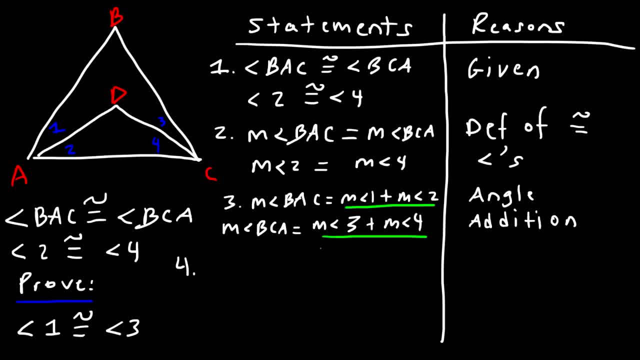 the measure of angle 1 plus the measure of angle 2 is equal to the measure of angle 3 plus the measure of angle 4, because they equal to these two things, which are equal to each other. So the measure of angle 1 plus the measure of angle 2 is equal to the measure of angle. 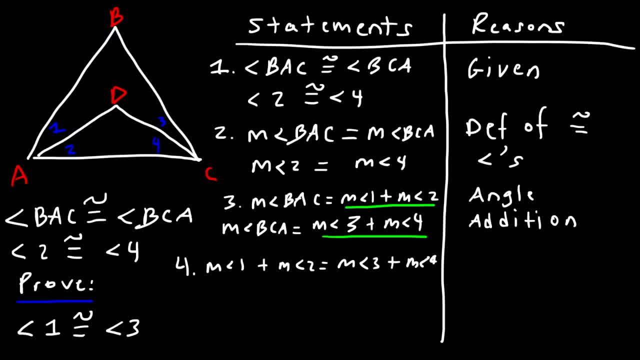 3 plus the measure of angle 4.. And so this is based on the substitution property. Now notice that angle 2 is equal to angle 4.. So therefore, we could subtract these two angles from both sides, because they're equal to each other.